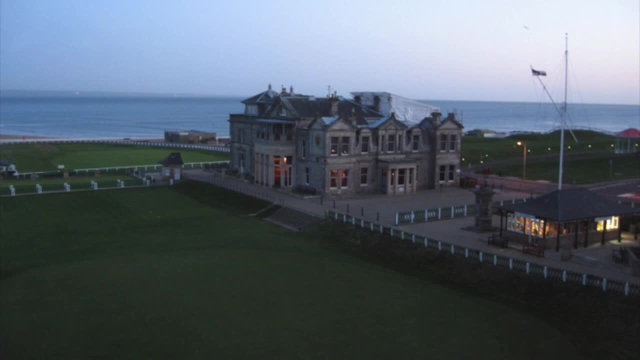 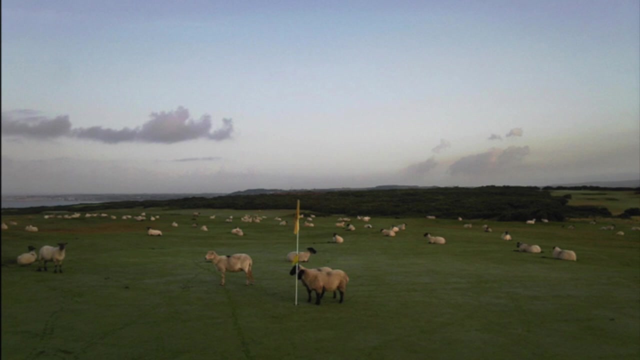 a book he was writing that he came across a Green's Committee minutes or report where the point of discussion during this meeting was focused on whether they should replace the sheep who were grazing the golf course. The concern was: did constant grazing dull or wear down the teeth, causing a lack of a clean cut by these sheep? I don't think. 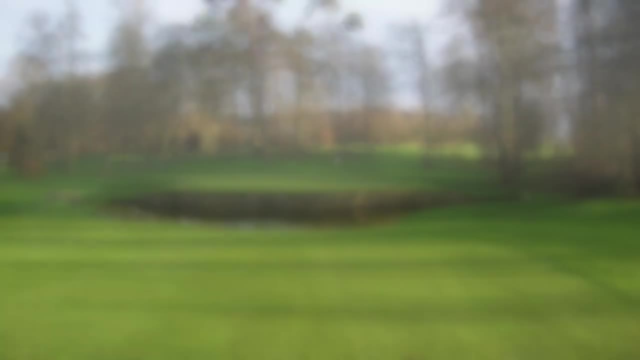 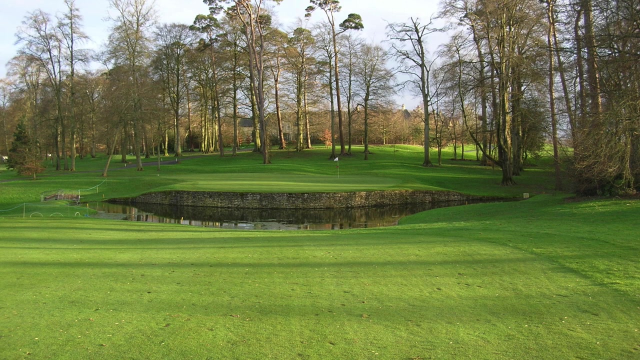 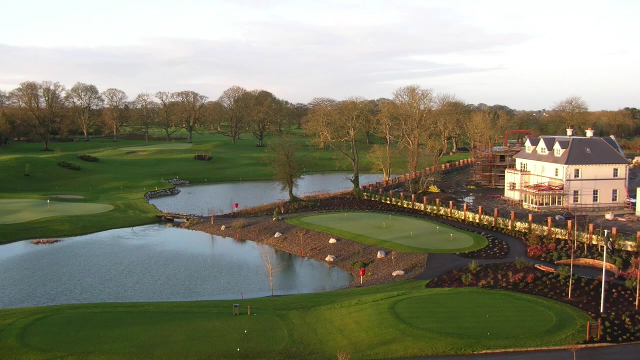 that's what happens, but anyway, As golf moved inland and golf courses were constructed on clay soils versus sandy soils that were present along these lynx or coastal golf courses, major detriments arose to playing golf with one of those with the presence of earthworms. These earthworm infestations resulted. 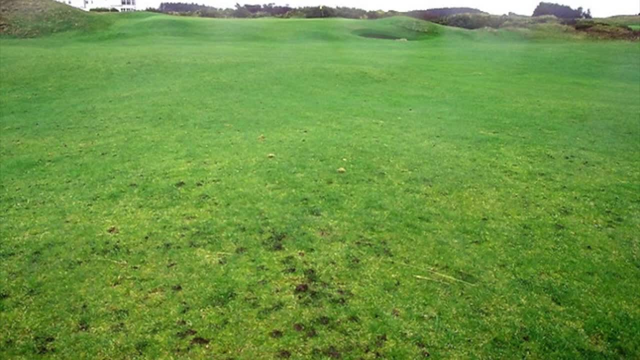 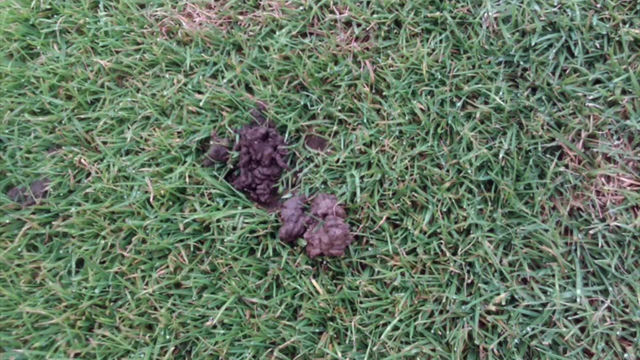 in numerous earthworm casts made putting greens unplayable for a majority of the year. During this time in the United Kingdom, organic and inorganic compounds were identified in the golf course that acted as either an irritant of the earthworm, causing them to emerge. 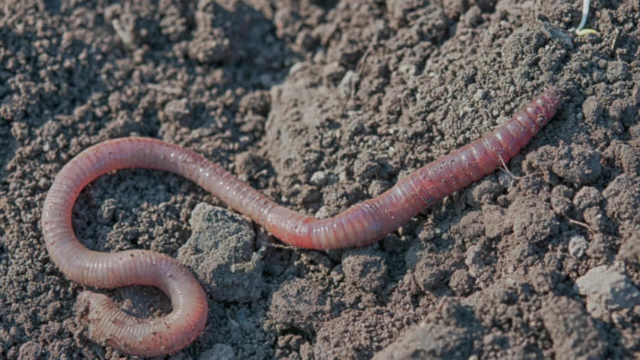 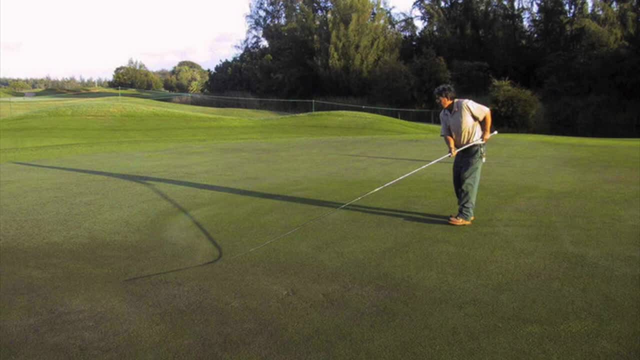 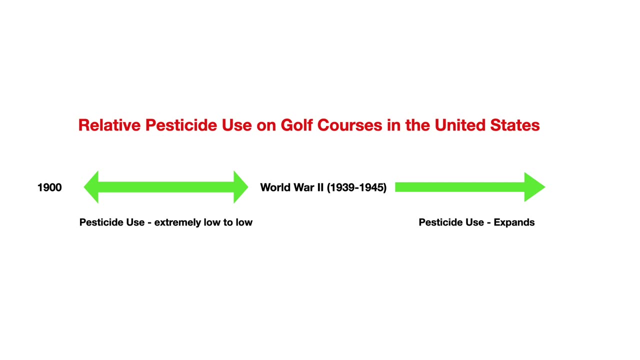 at the surface where they could be physically removed by crew workers on the golf course, or some of these compounds acted as being toxic to the earthworms. Pesticide use on golf courses in the United States can be divided into two general eras: Very few pesticides. 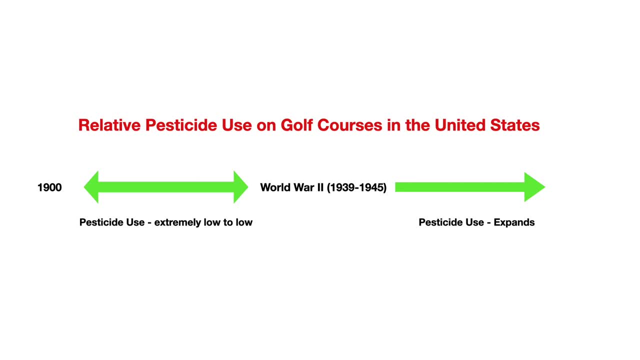 were used on golf courses in the United States, and very few pesticides were used on golf courses prior to World War II And then after World War II and into the 1960s, there was a large growth in the number of plant protectants used. 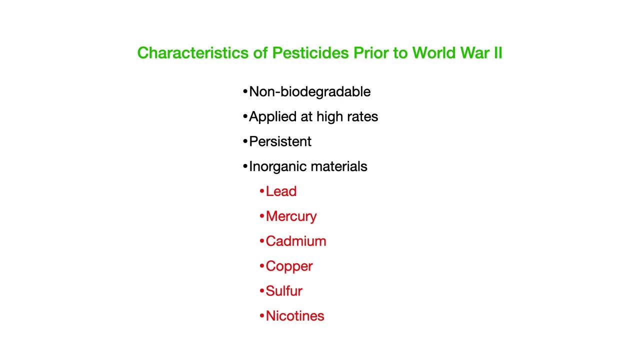 Many of the pesticides used from the 1920s to 1960 were characterized, as shown here, as non-biodegradable, applied at high rates, persistent and for inorganic materials containing compounds like arsenic, lead, mercury, cadmium, copper, sulfur or nicotines. These compounds 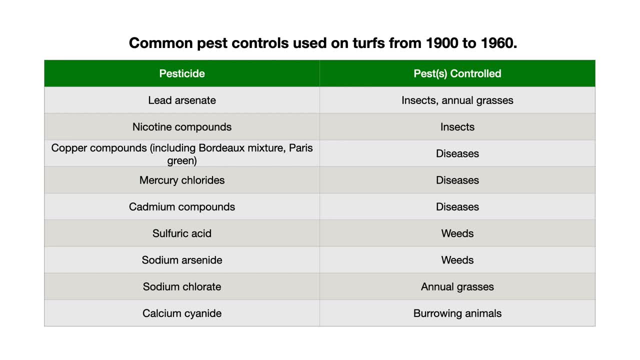 were known for their toxicity to humans. Many of these inorganic compounds had a broad spectrum use, And I'm not talking about just controlling turf diseases, for example. When we think of broad spectrum, we may think it controls multiple fungal diseases on a golf. 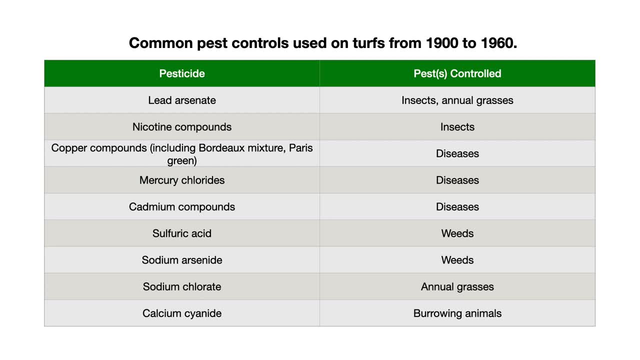 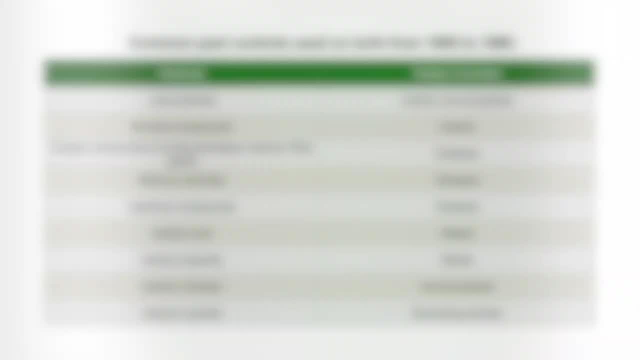 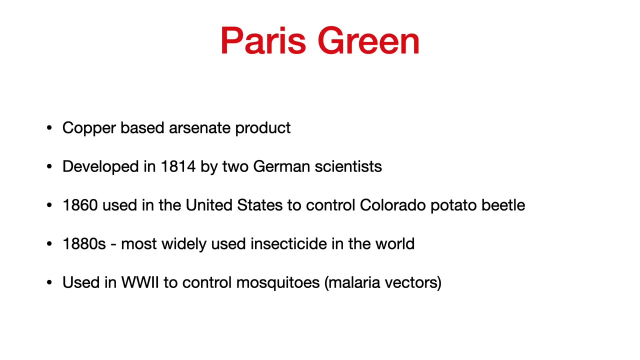 course, But back in the day with these products, these products had a broad, what I would call a real broad spectrum use. For example, Paris Green, a copper-based arsenic product, was developed in 1814 by two German scientists. It had some real poisonous. 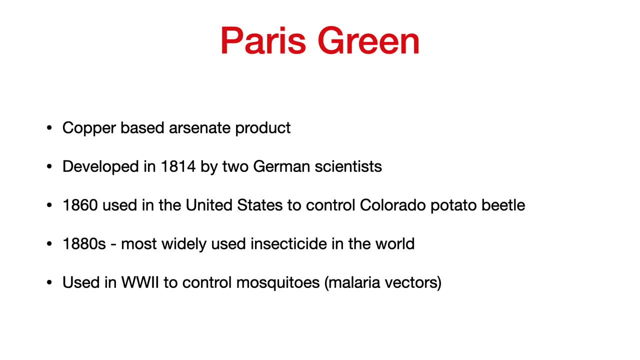 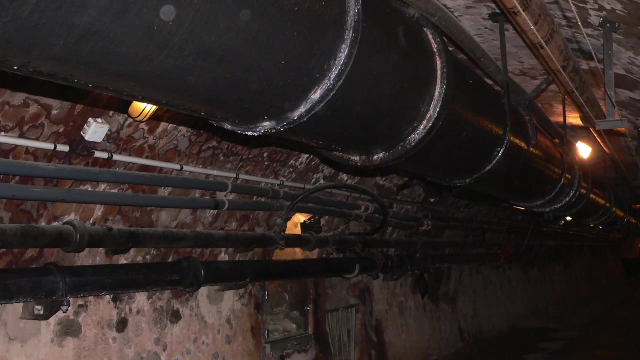 effects. In the 1960s it was used in the Midwestern United States to control the Colorado potato beetle in agriculture. In the 1880s it was the most widespread insecticide in the world. During World War II in Italy, Paris Green was widely sprayed to control malaria. 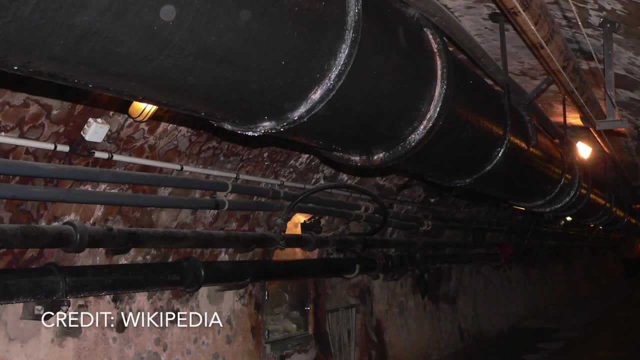 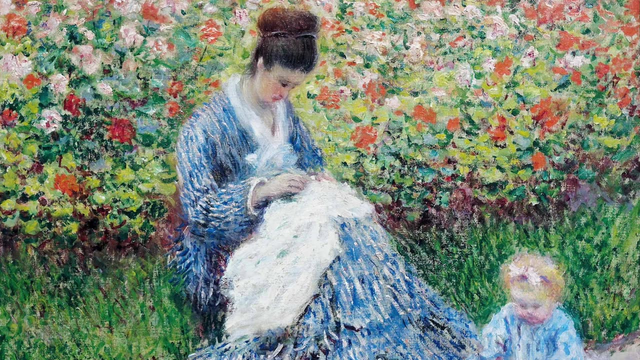 Paris Green gets its name from being used once to kill rats in the Paris sewers. Paris Green was also used as a pigment in paints by many artistic painters, including Monet, Renoir and Van Gogh. I probably would not have licked those paintings, but it gives you an idea of how widespread 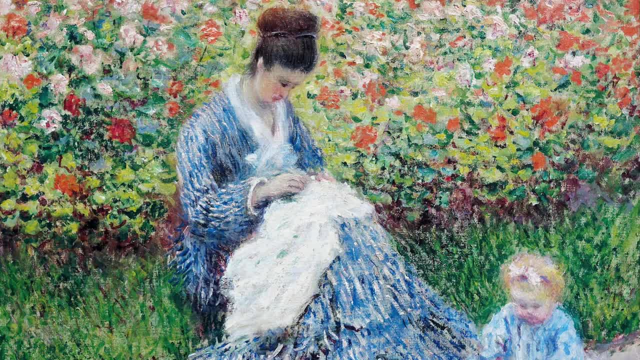 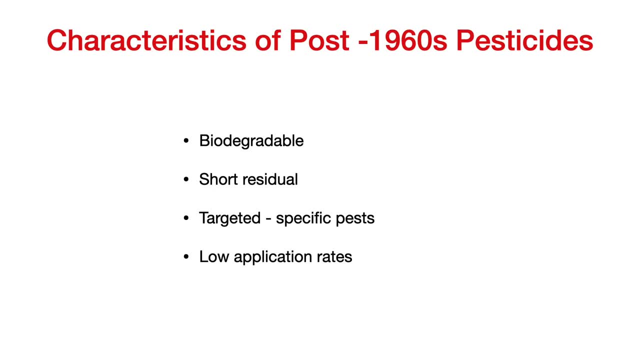 some of these toxic compounds were found in the cultures of the time. Starting in the 1960s, less-risk pesticides were developed that were one biodegradable, two characterizing by short residuals and low application rates, and organic pesticides specific to individual. 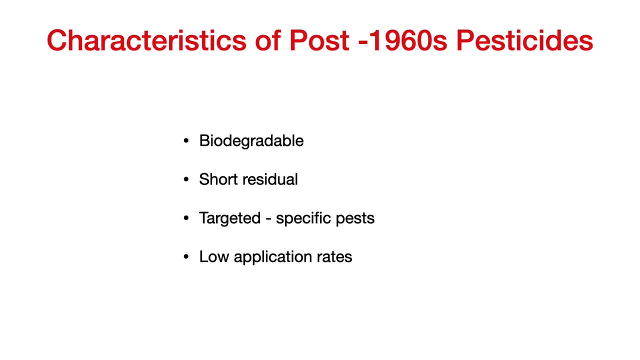 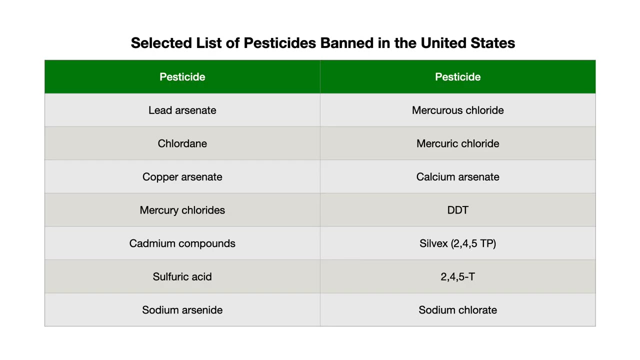 pests, thereby avoiding the use of broad spectrum. Short residual chemicals were a characteristic of these products, which meant they didn't persist for more than one growing season. Due to the development of newer pesticides, many of these older innovative pesticides saw a drastic drop in their use prior to the 1980s, when many like the arsenics were